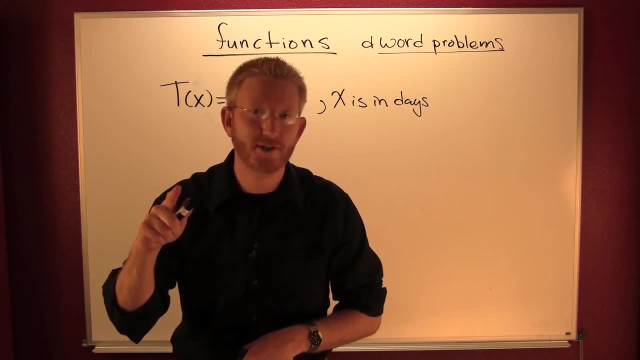 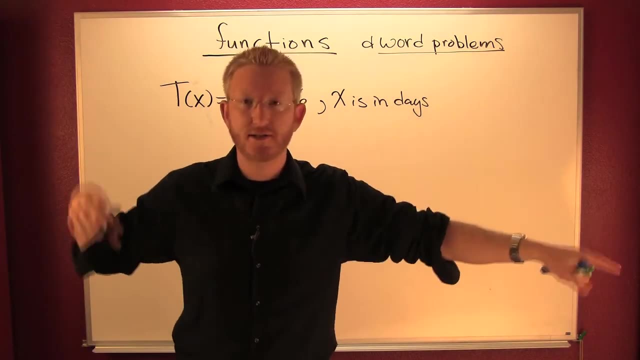 in like two weeks And then you'd be like 14 days, so I'm going to put a 14 there. That's all we're doing. What did I do? I removed the words Why To demystify these word problems They give you. 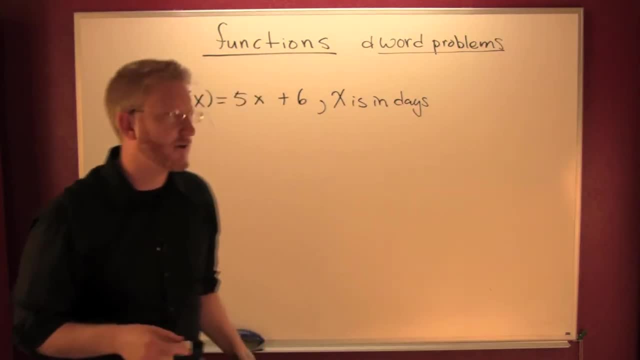 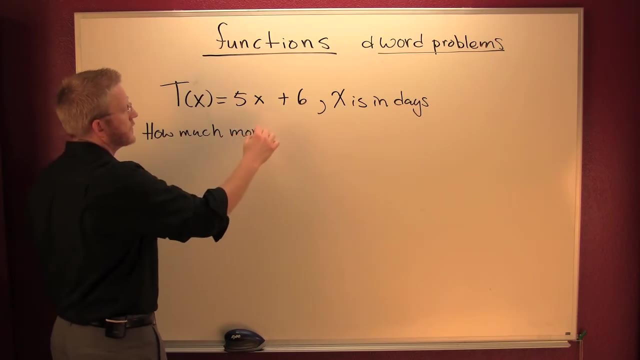 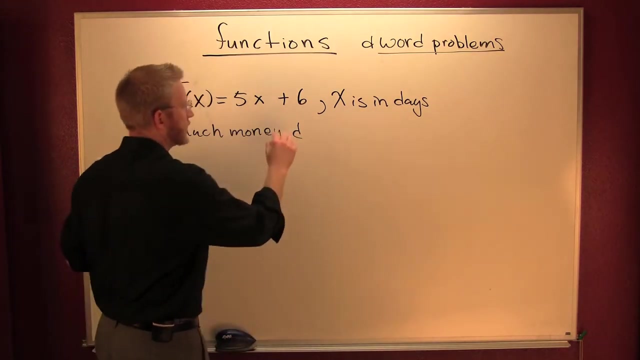 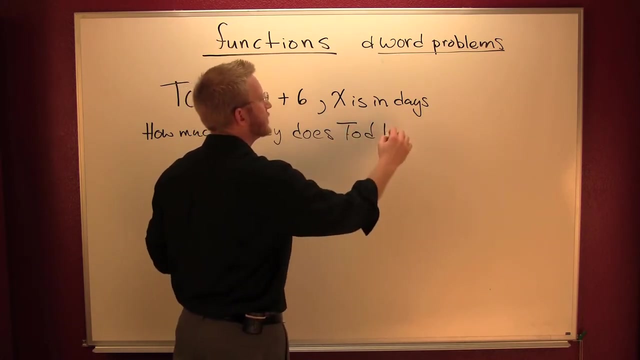 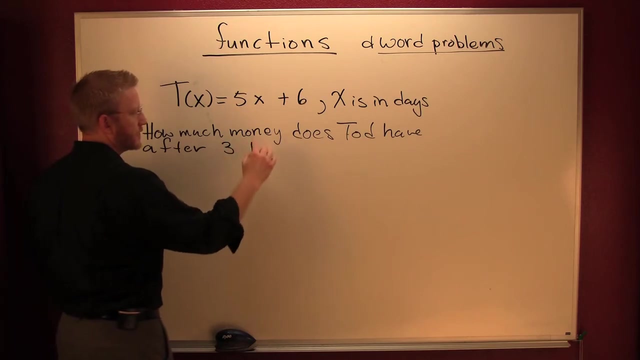 a function. Okay, You got to figure out where to evaluate that function Here. How much money does Todd make? Todd, Is that how you spell Todd? Ah, capital T Yeah, Have After Three days? Sure This. 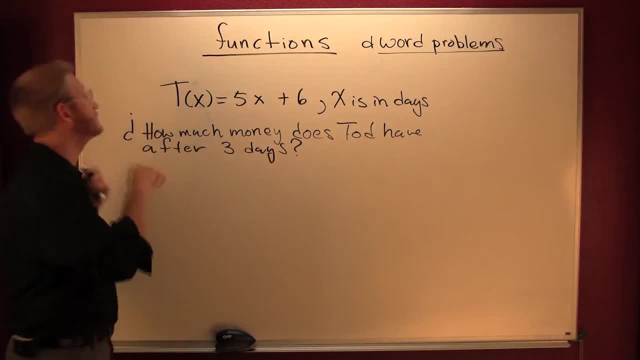 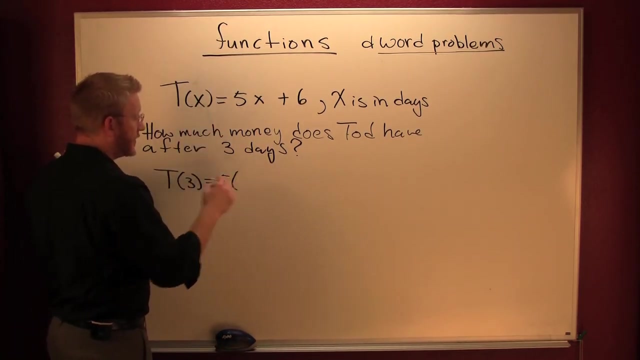 is the question: Good, scratch, Yeah. What are you going to do? You're going to find how much money Todd had after After three days, Yeah, And you're going to plug it in. Plug it in Everywhere you see an x. you're going to put a three T, Yeah, So then that's 15 and six Todd had. 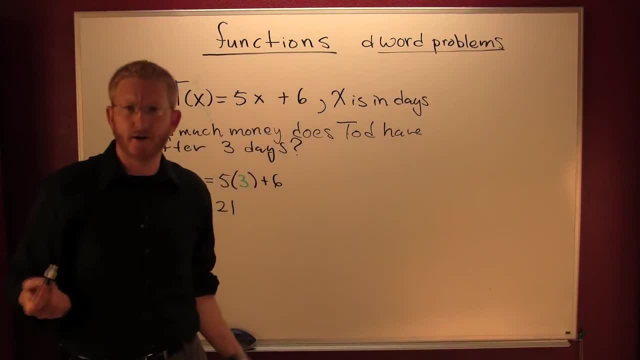 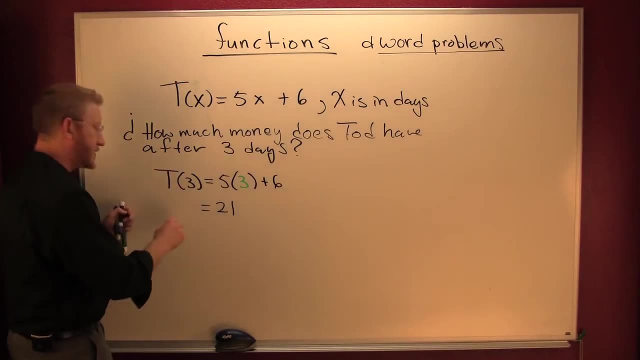 21 bucks, Right, Good stuff. Look at Todd Balling. And then, of course, you would write it up in a sentence: Todd had 21 dollars after three days. Uh-huh, All right. So I was saying that they coded sometimes. Maybe they want to know how. 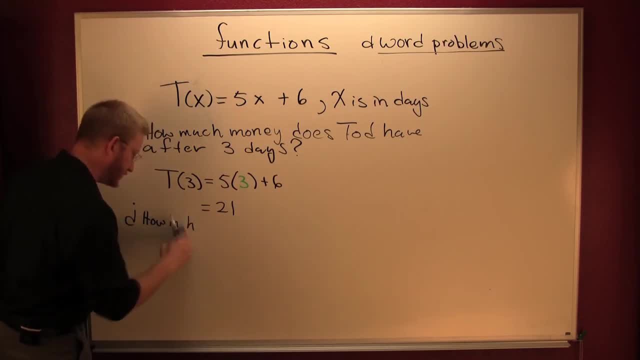 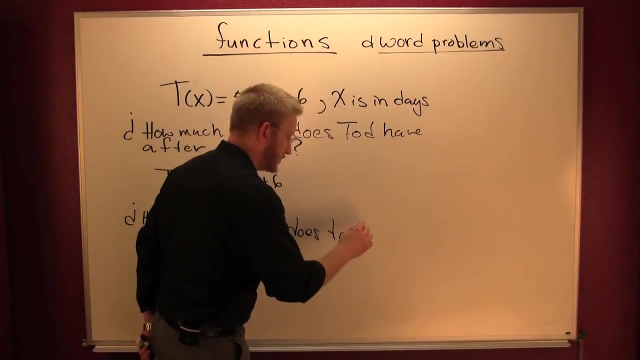 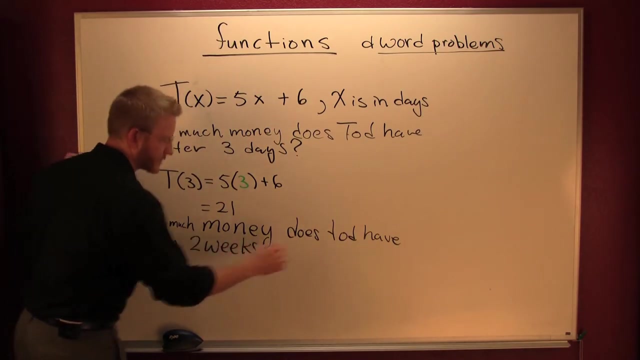 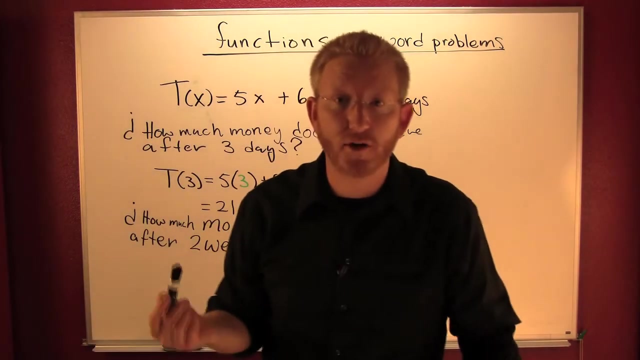 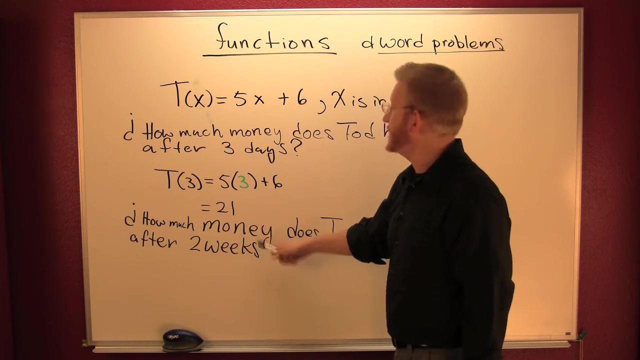 much. How much money does Todd have after two weeks? Woo Yeah. Well, how are you going to do that? Your function doesn't take weeks, Your function takes days. So what you need to do is you need to convert your x values from weeks into. 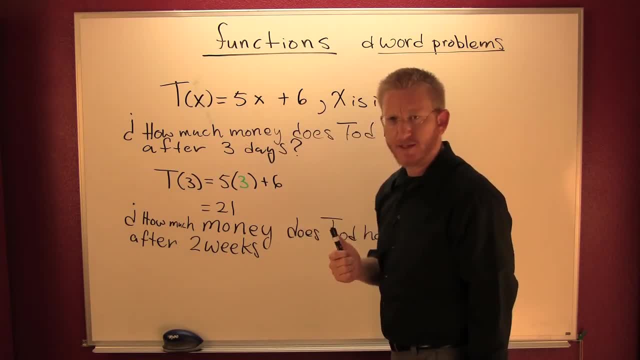 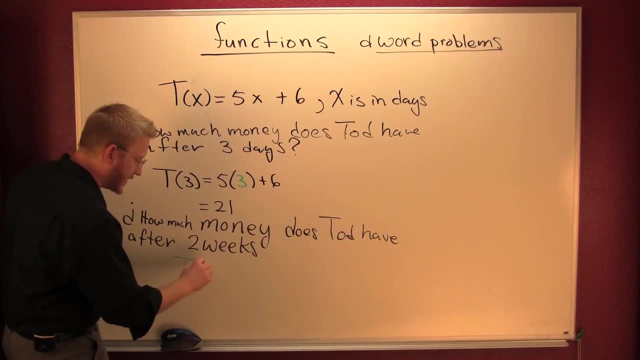 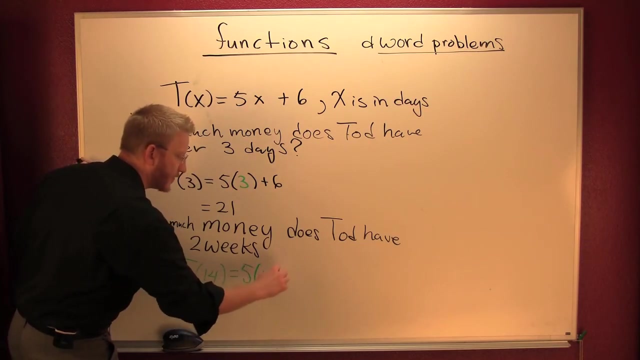 days, You got to ask yourself how many days? That's right, You're going to let x be 14.. So we want to see how much money Todd has after 14 days. Yeah, So this is five times 14 plus.